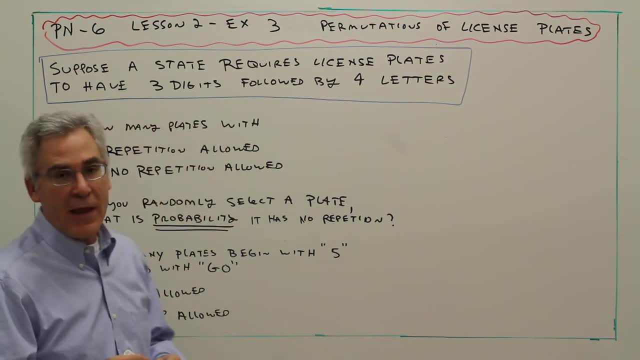 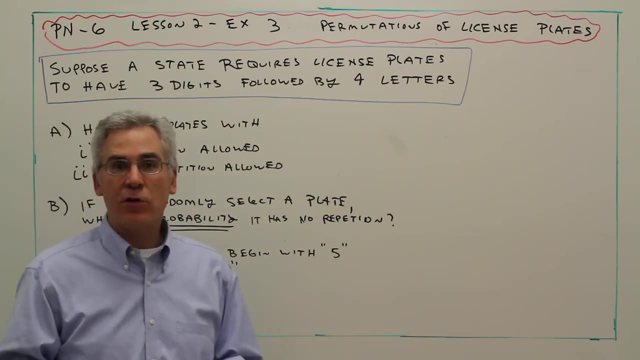 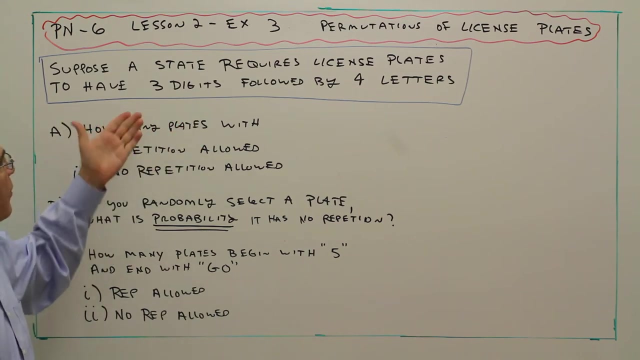 Welcome to video PN-6.. This is similar to Lesson 2,. Example 3, Permutations of License Plates. Here's the problem. Suppose a state requires license plates to have three digits, 0 through 9, followed by four letters, and each letter could be A through Z. 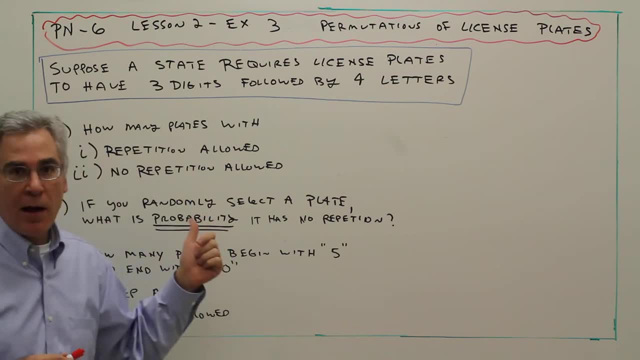 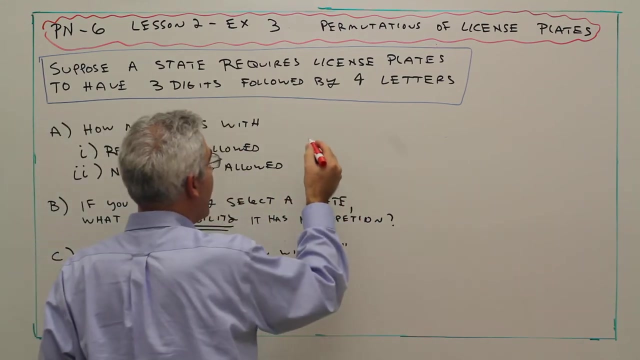 Several questions. First one: How many different plates are possible with repetition allowed, repeating digits or letters, and then, in the second case, without repetition allowed. So we'll do the first one here. I'm a visual person, so I like to slide it up. 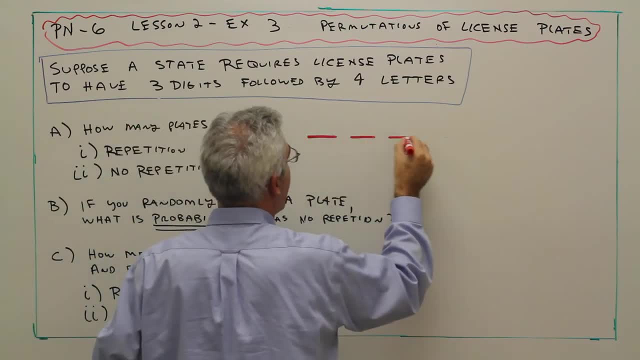 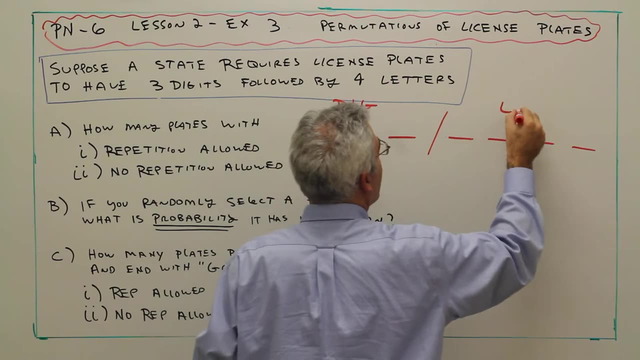 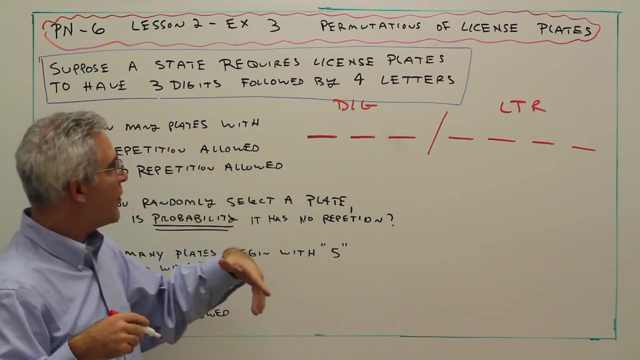 So three digits. I'm going to make three blanks. So these are the digits and these are the letters. Okay, and we're doing this first example here. Alright, with repetition allowed. well, this could be anybody from 0 through 9, 0 through 9, 0 through 9.. 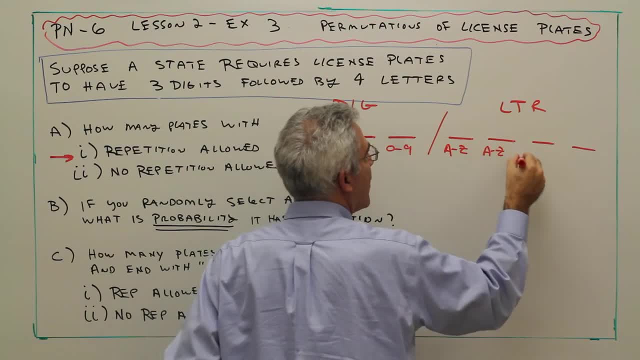 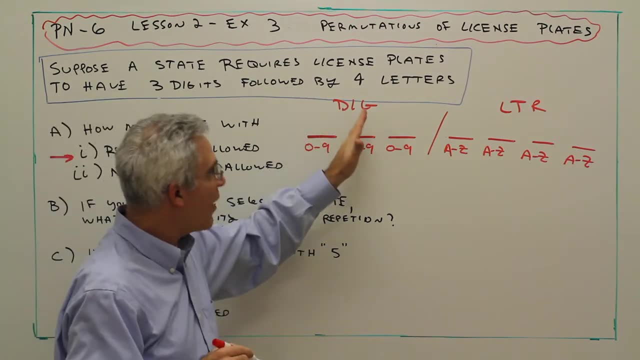 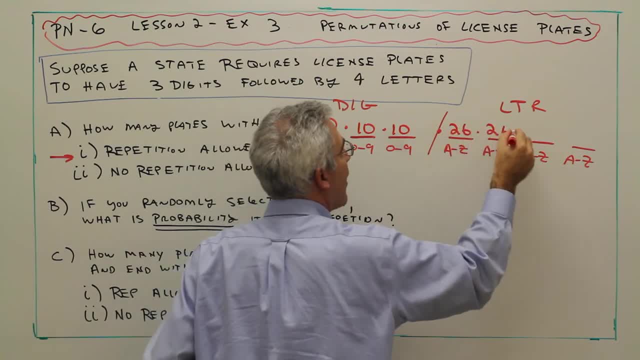 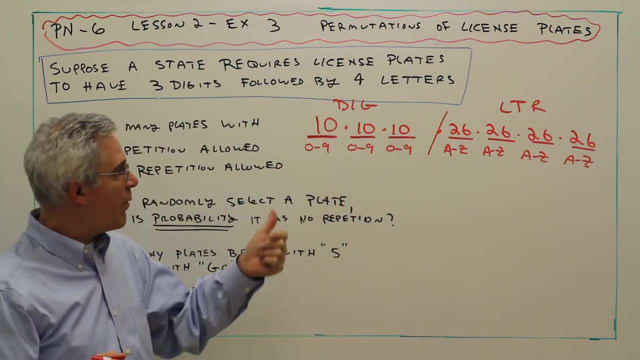 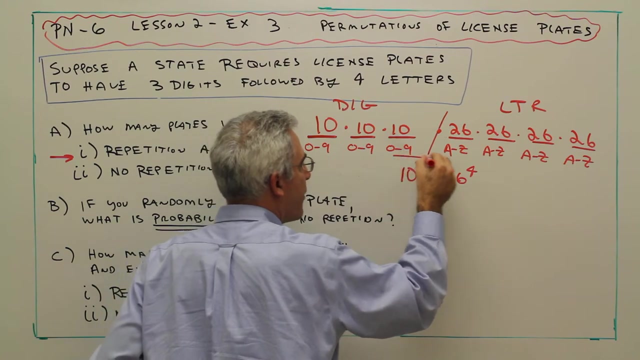 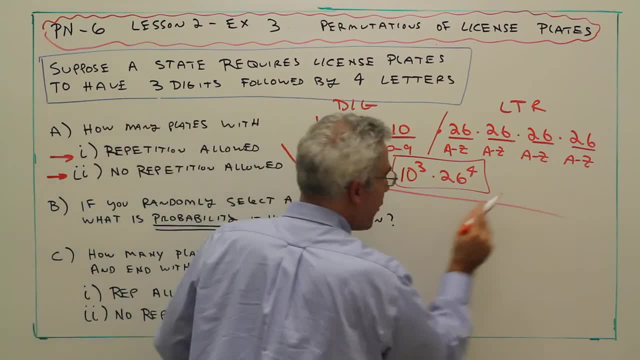 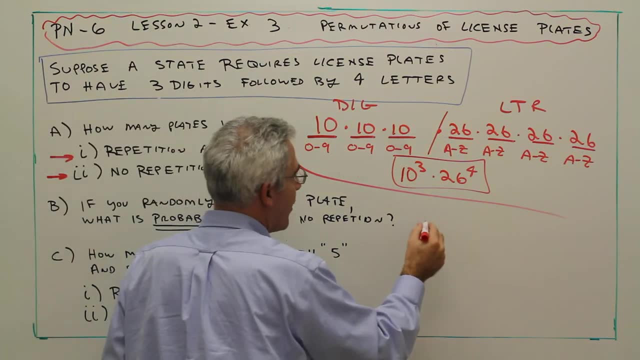 Alright, now we're going to do the second part. I'll do that below here. then I'll erase How many are possible, with no repetition allowed. Alright, so again: 1, 2, 3, 1, 2, 3, 4.. 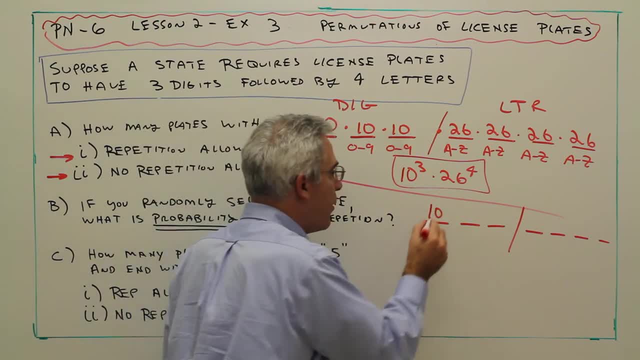 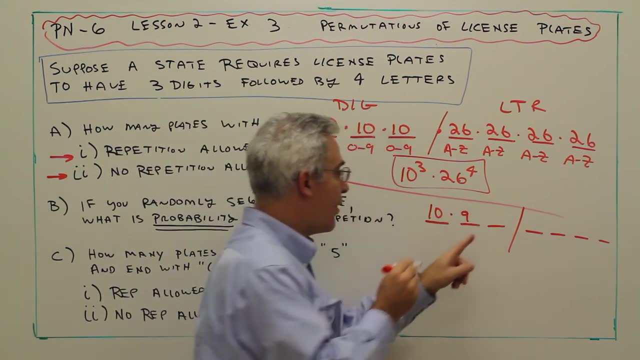 Alright, so I could put any of the 10 digits here, but once I select a digit there, I can't use it again, So there's only 9 left to choose from. Likewise, over here, I can't use that digit or that digit, so I've only got 8 to choose from. 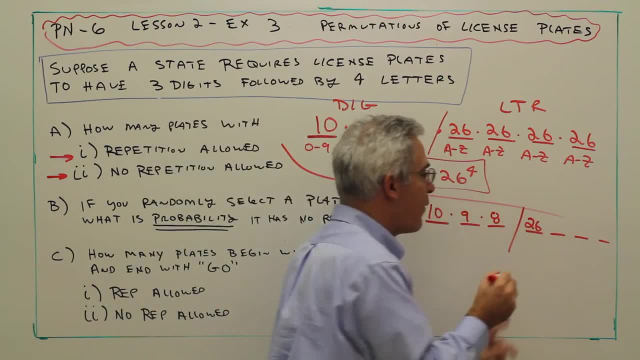 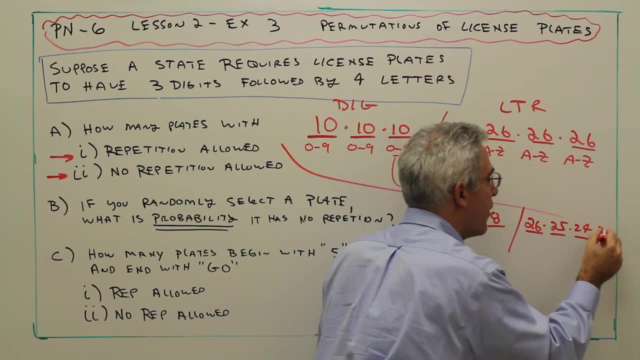 Okay, for my letters again I've got 26. For my second one, I can't repeat 25,, 24, and 23.. And for this video I'll just leave it like this. You could multiply it out. 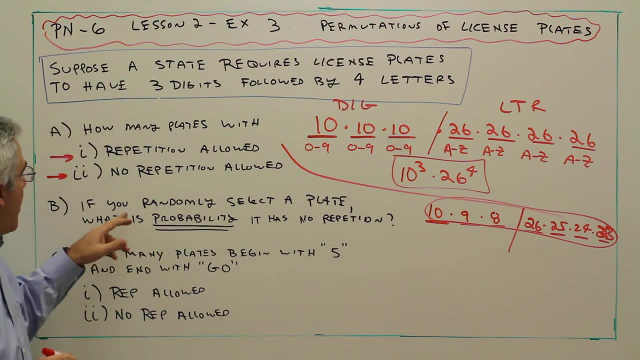 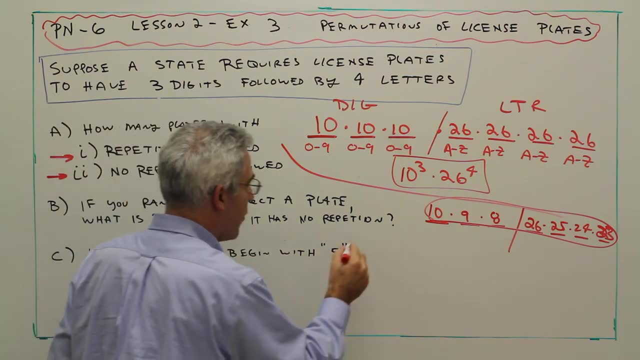 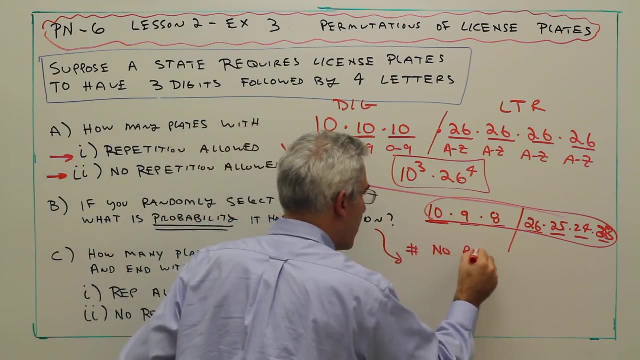 Okay. problem B: If you randomly select any license plate, what's the probability that it has no repetition? So I'll put that. Okay, I'll put that work over here. So it's the number with no repetition over the total. 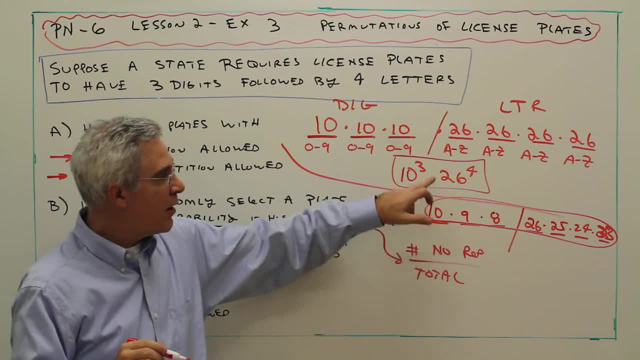 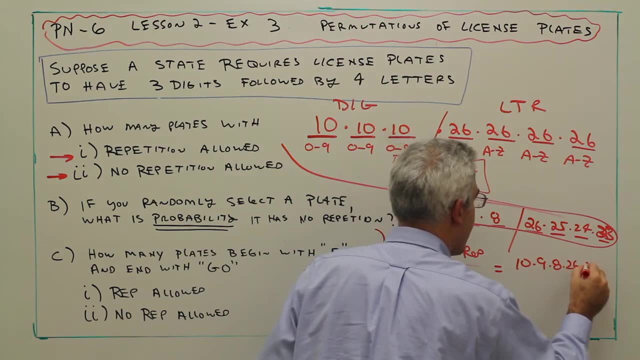 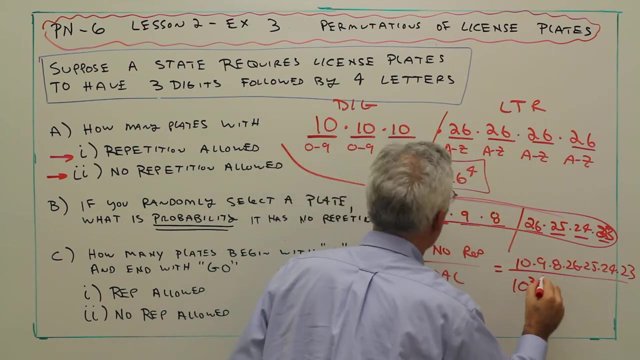 Oh, this is the number with no repetition. This is the total, So it's going to be 10 times 9 times 8 times 26 times 25 times 24 times 23.. All over 10 cubed times 26 to the 4th. 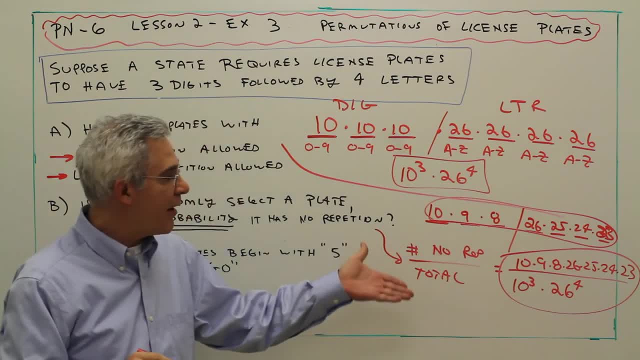 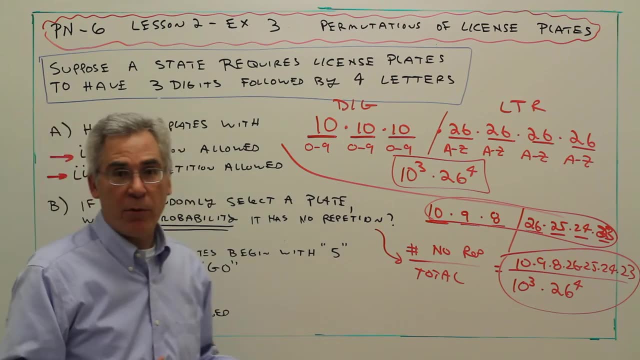 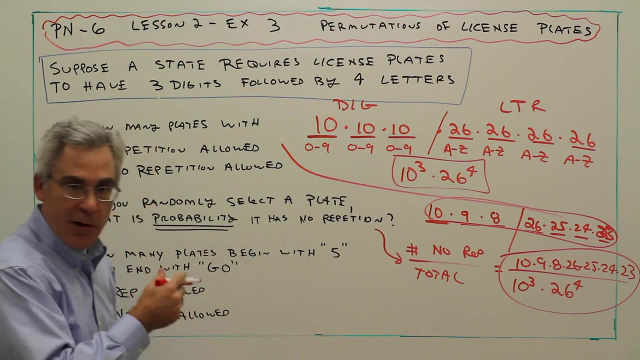 And again, you could calculate that with your calculator, but just for this video I'll just set it up for you. Typically we'll give three decimal places for the probabilities. Okay, and then finally, let me erase this work here. 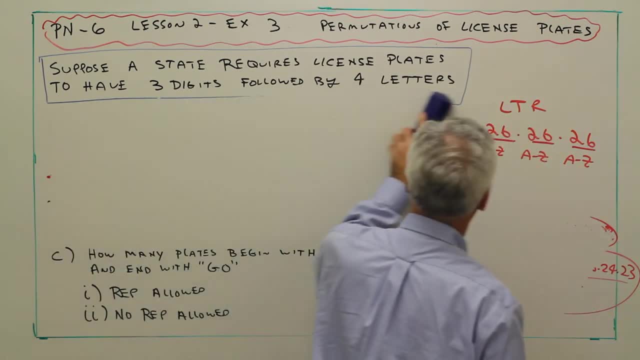 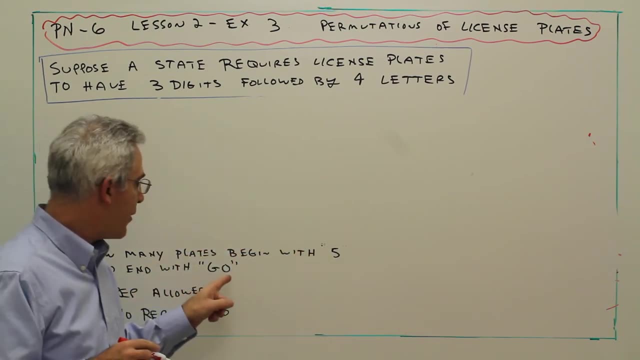 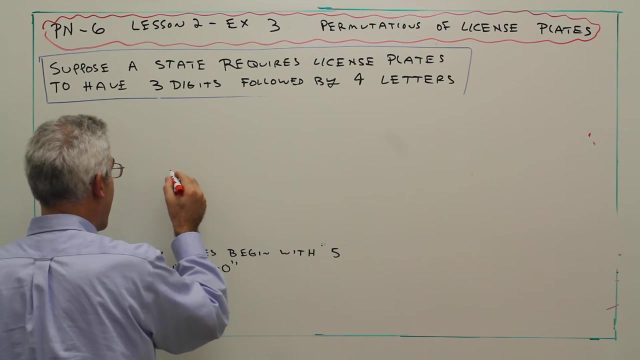 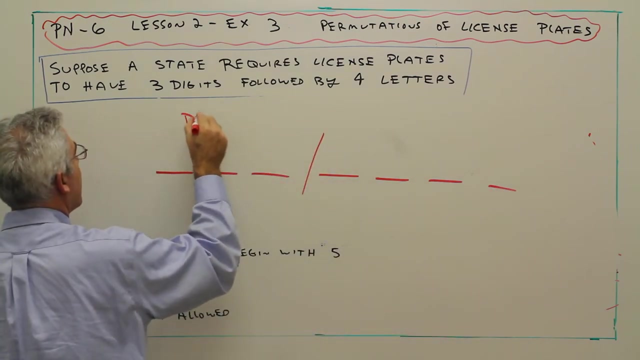 Here: How many plates begin with the digit 5 and end with the letters G, G, O, my initials, with repetition allowed and without repetition allowed. Okay, let's set it up again. So these are the digits, These are the letters. 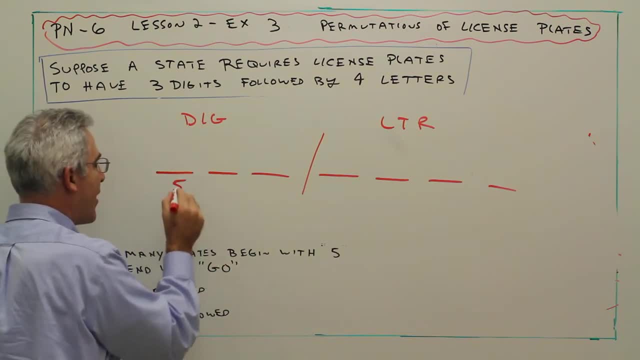 So it says it must begin with the digit 5 and it must end with G O. So I just kind of put what the possibilities are below. Well, there's only one way of doing that, There's one way of doing that, and there's one way of doing that. 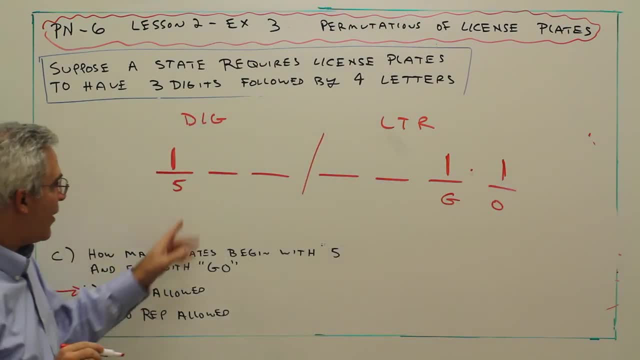 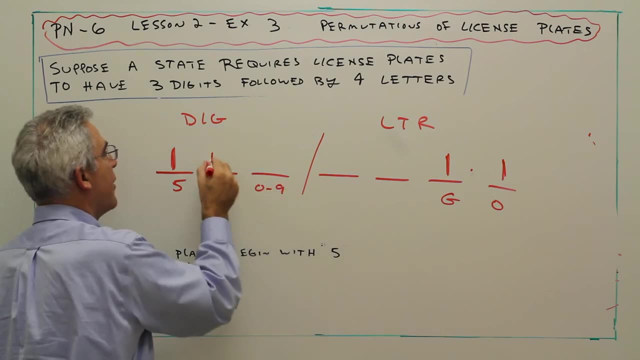 All right, so we're going to do it with repetition allowed. So over here I can repeat the 5.. Again, it could be anybody: 0 through 9,, 0 through 9.. So there's 10 ways, 10 ways. 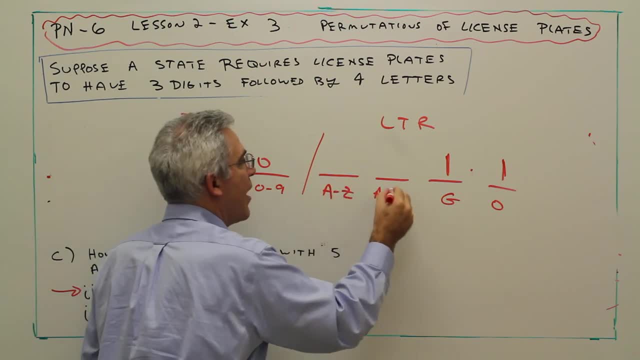 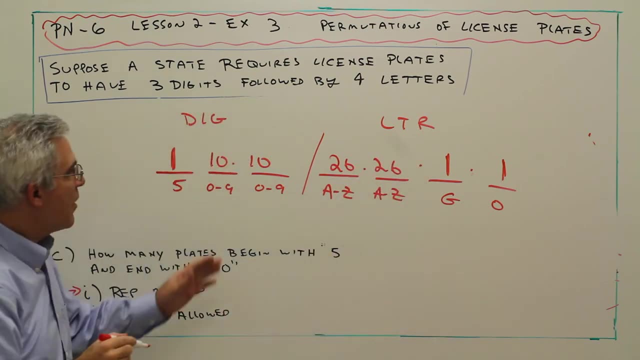 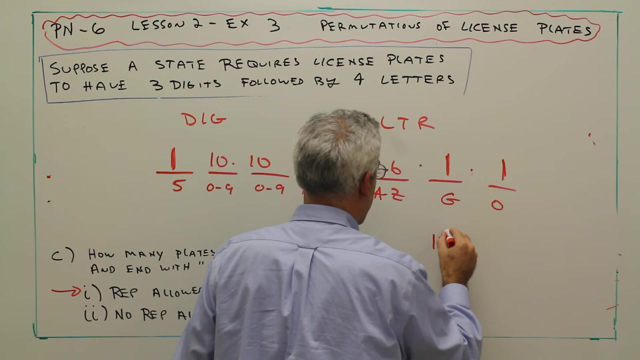 Over here. it could be anybody A through Z, anybody A through Z, So 26 times 26.. So my answer is So. my answer simplifies to 10 squared times 26 squared, And again you could calculate that with your calculator.